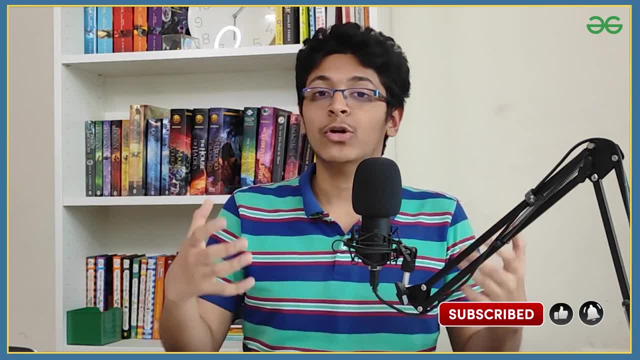 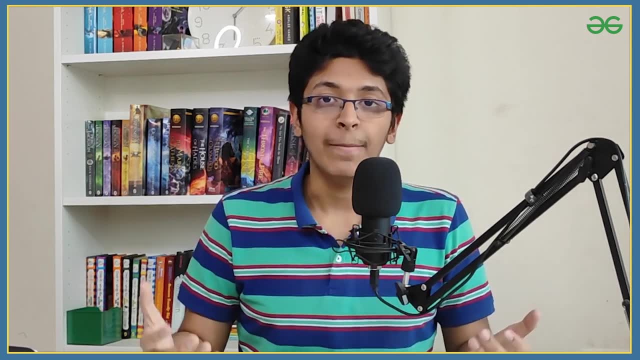 the steps that are required, what all code you need to type, what does that code really mean? and we'll also see the end result from there on. So first of all, let's talk about the requirements, the dependencies that will be there for you to install first of all. So first thing is going to: 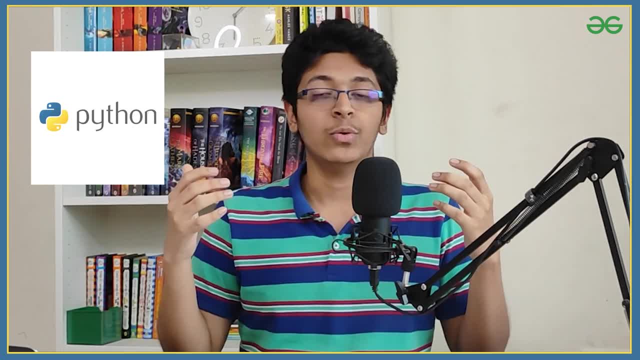 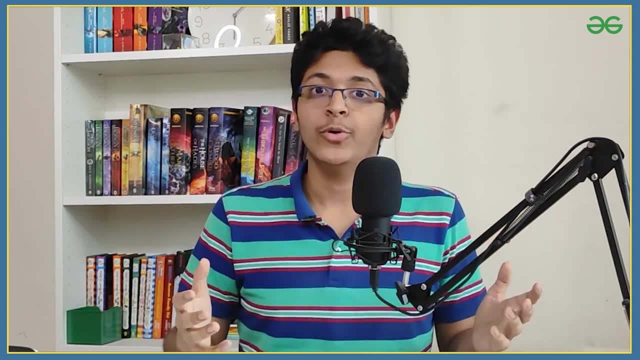 be Python. So we're using Python for doing this, and if you want to get started with web scraping, Python is a great language. Simply just go to pythonorg and you can install Python. I hope you can do that much After that. now I'll show you how can you get. 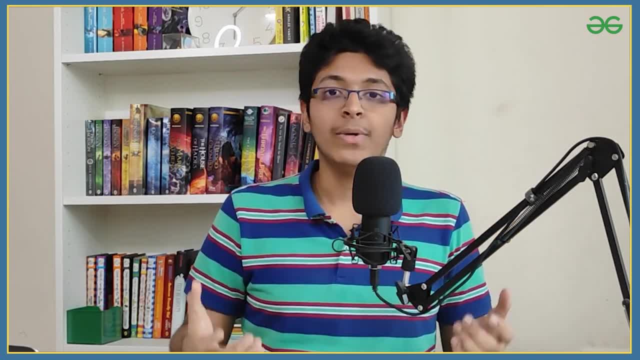 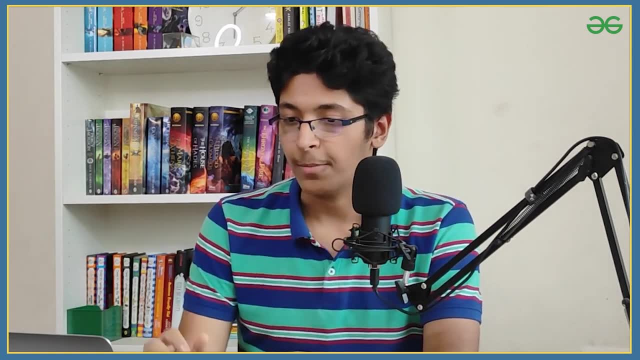 yourselves the three or two modules that will be required. Number one would be Beautiful Soup and the second one would be called as Requests. Okay, so now let's take a look at what all you need to do by going onto the laptop. Let's do this, Alright. so, as you can see, 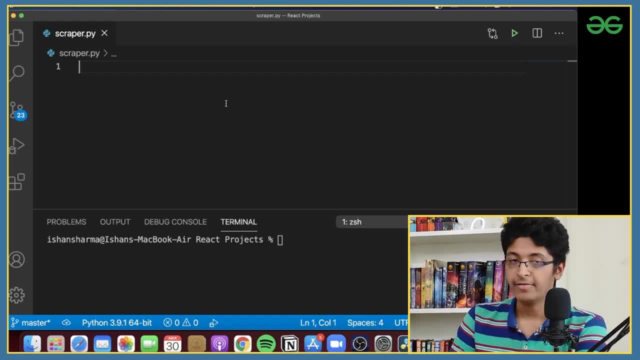 I have Visual Studio Code opened up and I have just made a file called scraperpy. Okay, that's the Python file that we'll be using. So, first things first, we'll need to actually get Beautiful Soup, Okay, so for that I'll just go on to my Chrome and I'll just search for. 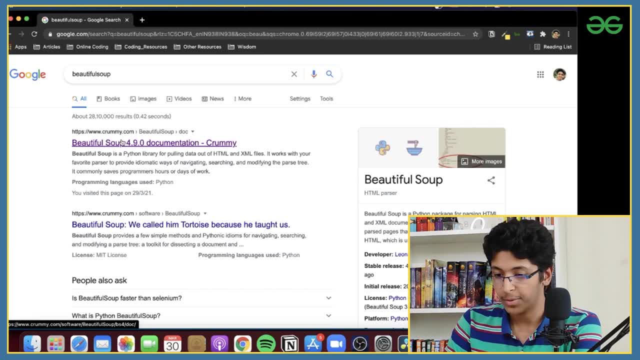 Beautiful Soup. and that is right there. This is the complete documentation Highly suggested for all of you to go through this. Okay, so let's get started, So, let's get started, So, let's get started. You can also look at our GeeksforGeeks blogs on this thing. But let's go back. 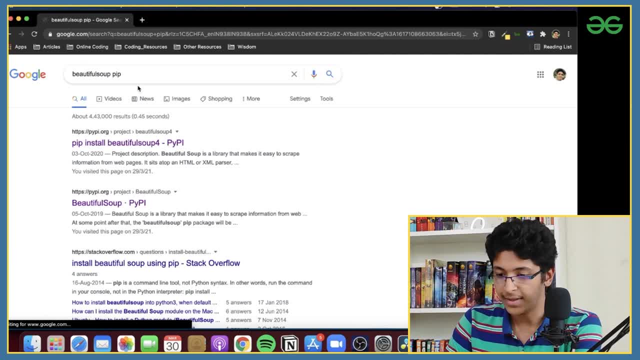 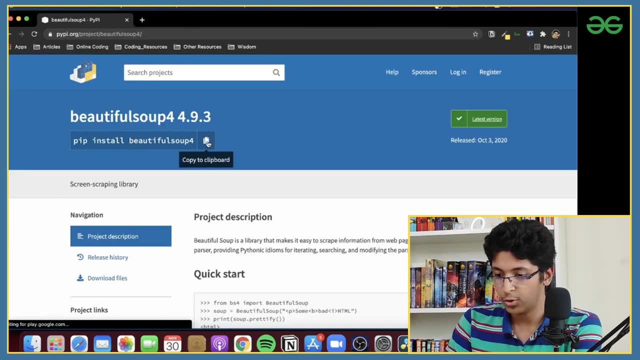 and let's look at how can we do this. So just search for PIP. that is pip, that is Python package installer. So after that we'll just click on this and we'll just need to copy this thing. Okay, so just just copy here, And once you've done that, we can open up our terminal. 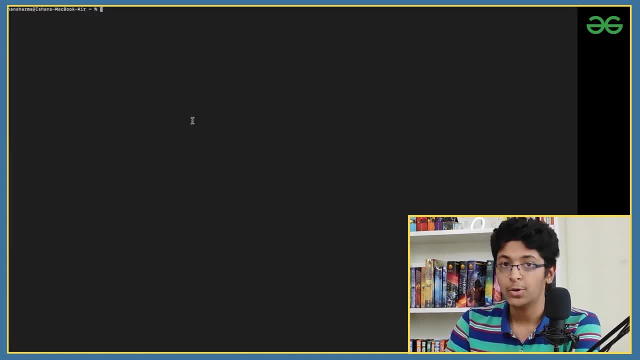 And on the terminal- let me just go full screen Here- you just need to type PIP three, PIP three, install And you can type the whole thing that they wanted you to do. And so I am using Mac, So on that I have to do PIP three, But if you are using Windows you can just do PIP And that. 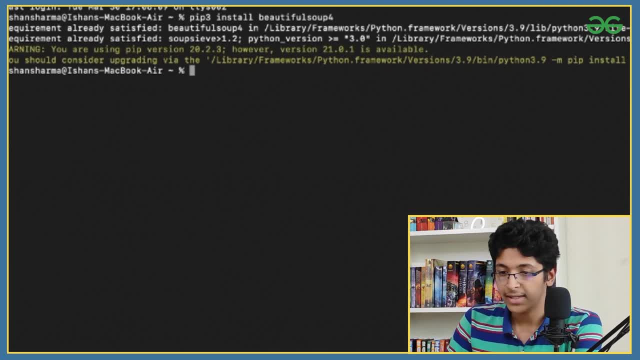 should work fine. for you just click on Enter And for me it says requirement already satisfied. So that means that I am good to go. Now let's take a look at how can we install the requests module. So first of all I'll just say: pip three, install. 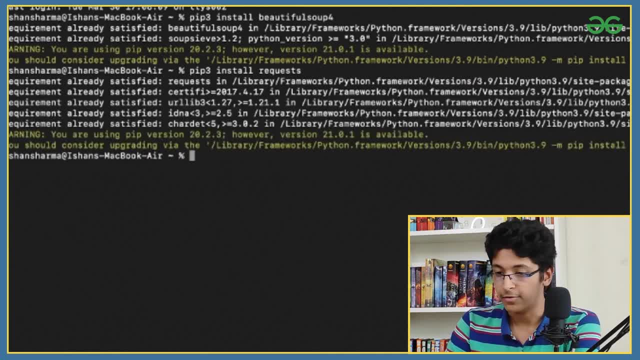 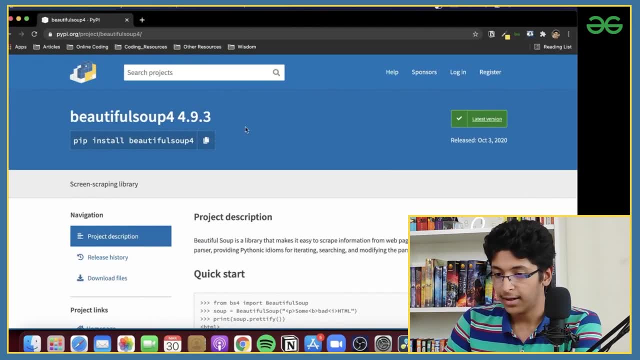 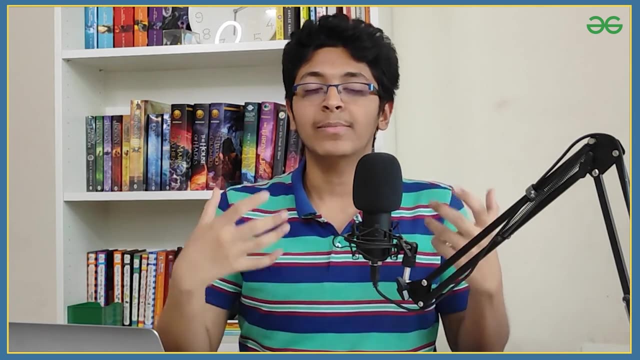 Request, I'll press Enter, And that is also satisfied for me. So now I have installed both of the you know modules that were required. Now let's go on and take a look at our file here. Okay, so what happens is that let's try to understand what is web scraping essentially? 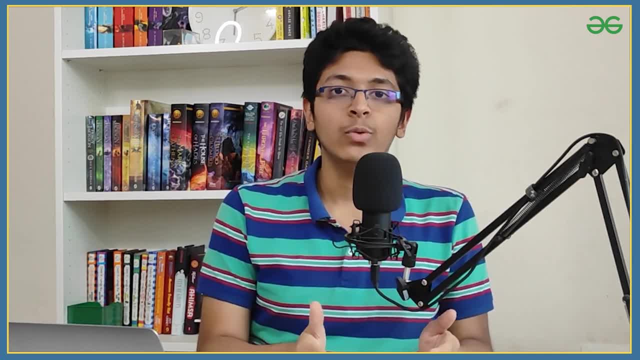 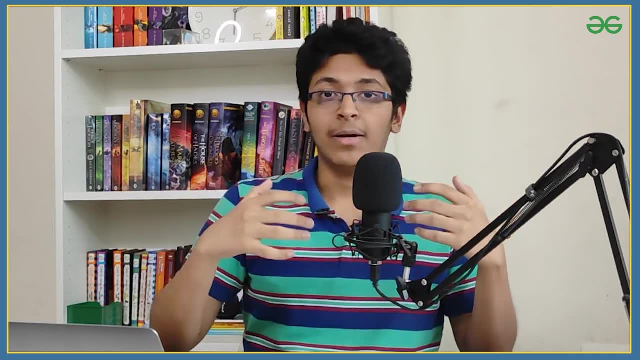 basically, we want to take some website and you want to scrape data from there. you want to take some information that you can use for your own purposes. Maybe you want to make like a, like a for some thing that you want to buy online, or or maybe you want to just see what the temperature is. 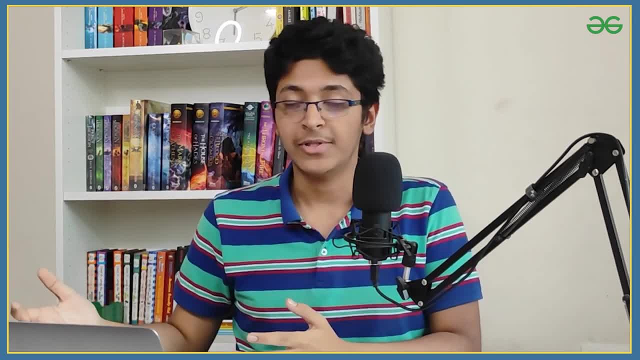 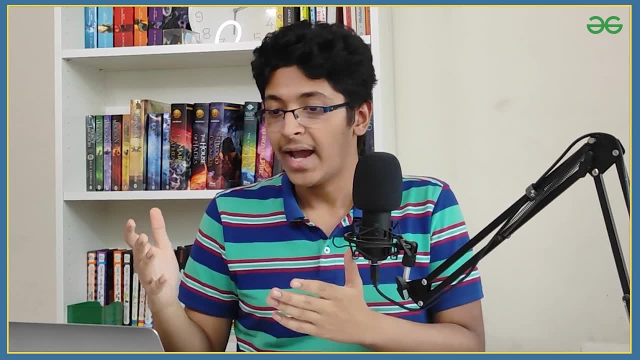 right now, Or maybe you just want to see the latest blog on a particular website, So things like that. if you want to do, and that particular service or website does not have an API, then you can go ahead and use something like this. But just keep this one thing in mind: that not all websites 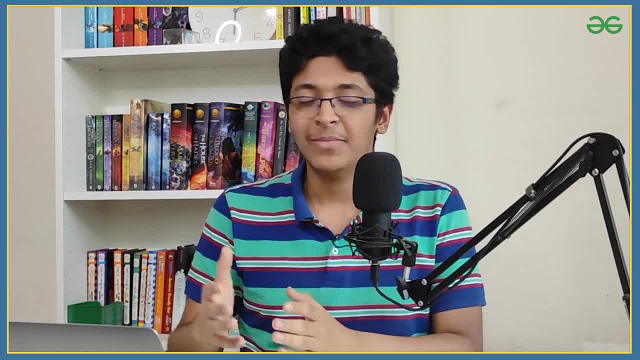 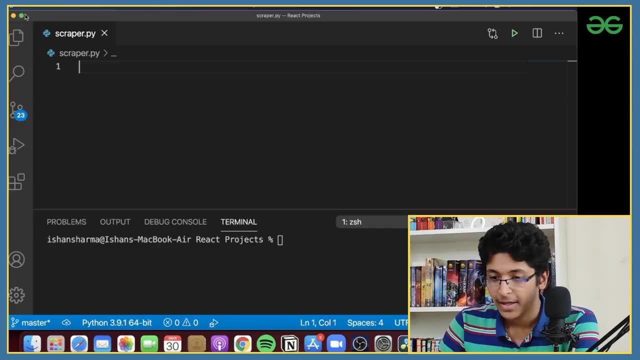 are happy when you actually scrape their website. So just keep this one thing in mind: make sure that your website that you want to scrape allows you to do the scraping. That's one thing to do, Keep in mind always. So now what I'll do? I'll just go full screen with this, And first of all, 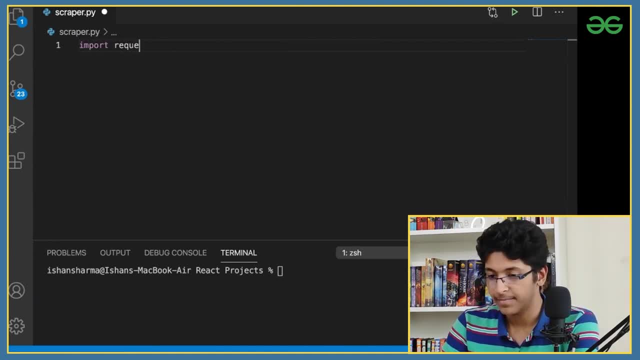 we'll need to import all of them. So I'll just say import requests And I would say from BS, for that is beautiful soup for import, Beautiful soup. So first of all, what I'll do is that I will get something called as a request, right? So, request for a particular website. I'll just 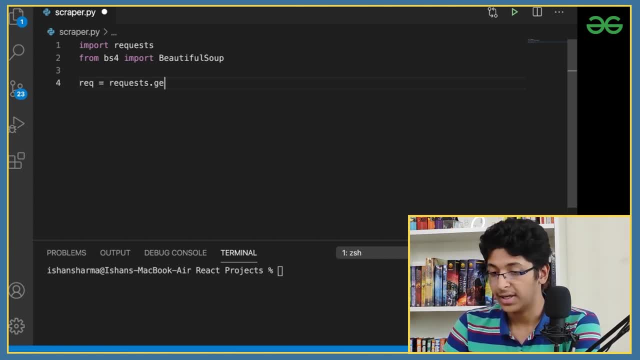 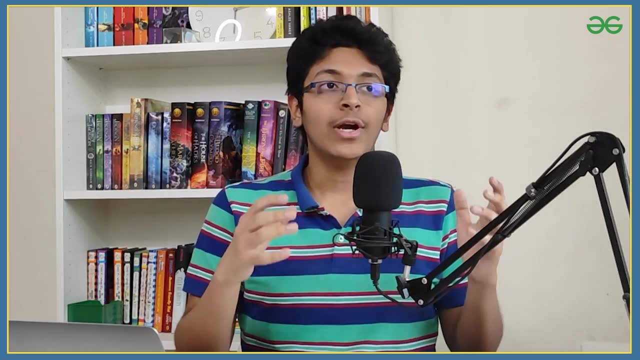 call it our EQ and I'll equate that to request dot get And I'll have these brackets And in between I'll need to put in the URL of the website. Now it is not really required that you have a website. you can also just link it to HTML document that you 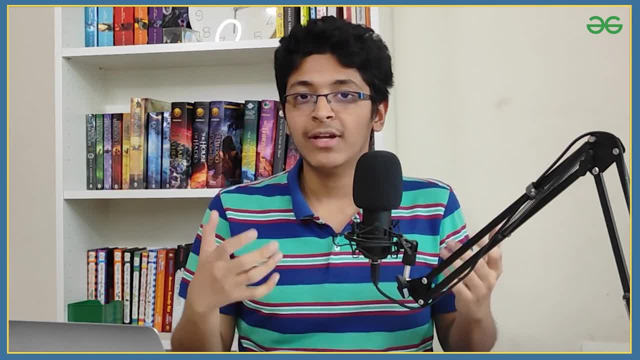 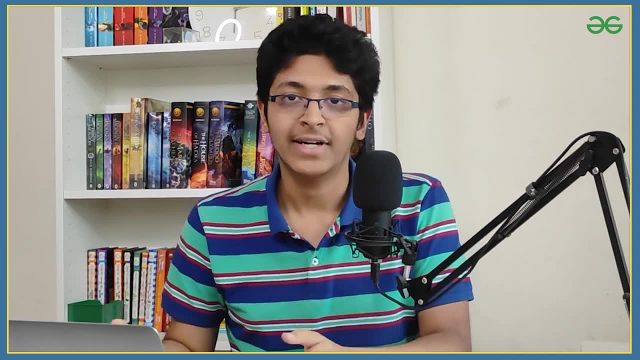 have in your own folder. But the thing is that if you are using web scraping, it is generally used for websites that are online and not on. you know, websites that are in your local folder itself. you can just go on. you can see whatever data is in it. But anyways, we will actually get some sort of 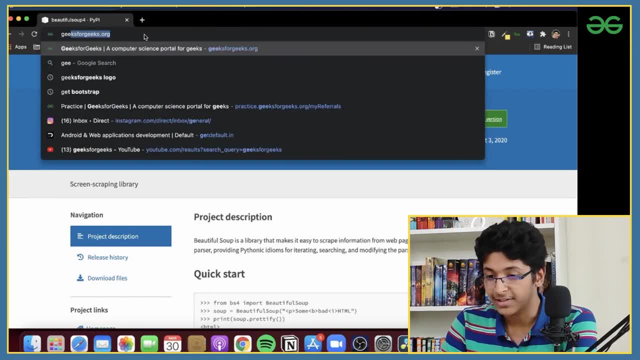 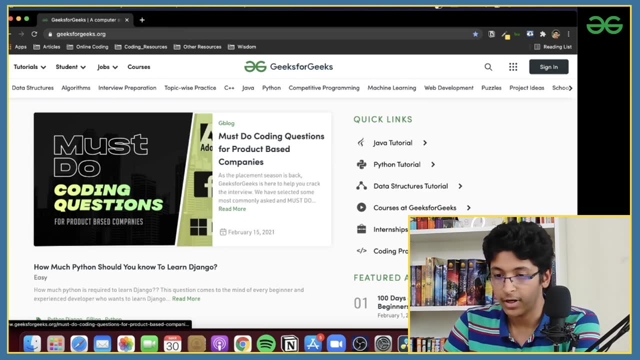 hasn't proven or received a ever. so I'll just go here and I will actually go to geeks for geeks. right, he's really start orgy And here what I will do is that let me just close all of this thing here and 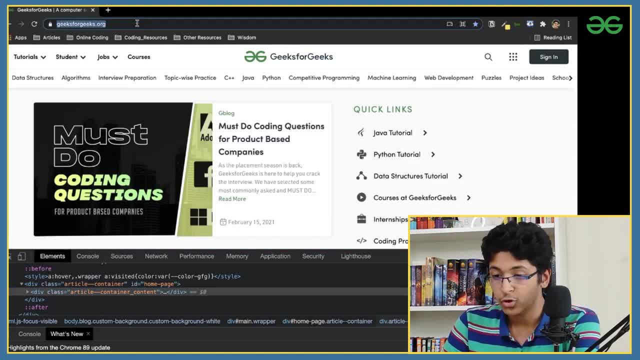 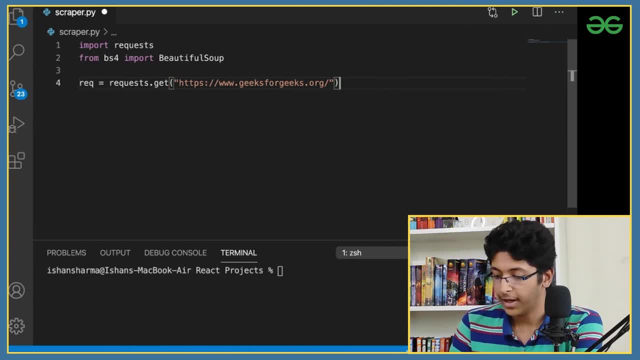 I will click on inspect. Okay, I'll click on inspect, but we'll do this afterwards. I'll just copy this link of keys for parts dot o, RG and I'll go back and paste this right here. Okay, So will do is that we will use something called as a soup and in this thing we'll just create an. 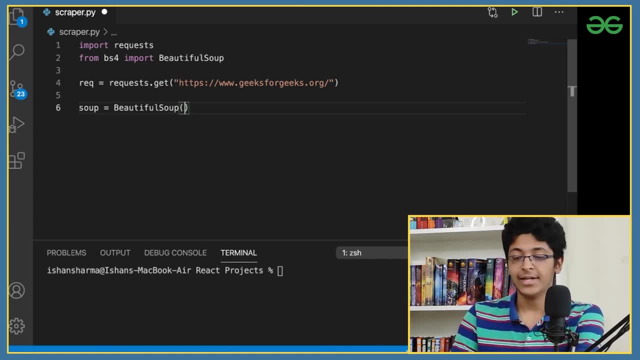 instance of beautiful soup. okay, so beautiful soup. think of it like a class that you have and you're just creating an object called a soup. so here i'll just say that, okay, i want to get the content from this particular website, so i'll just click on content and then i'll say that the parser that i 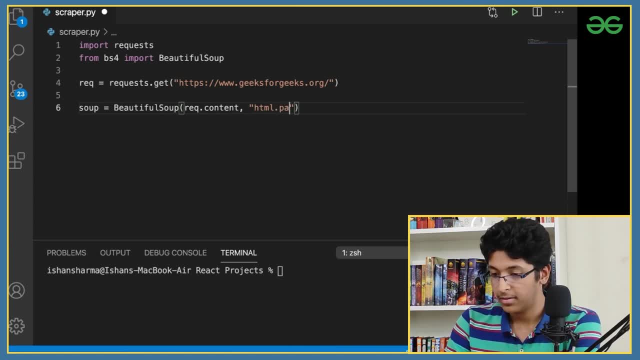 want to use is just going to be called as html parser. okay, so that's all that you need. okay, now, first of all, let's just see what this soup actually has, so i'll just print out: soup dot- prettify. okay, so this prettify is important, because else we'll just get some hodgepodge. 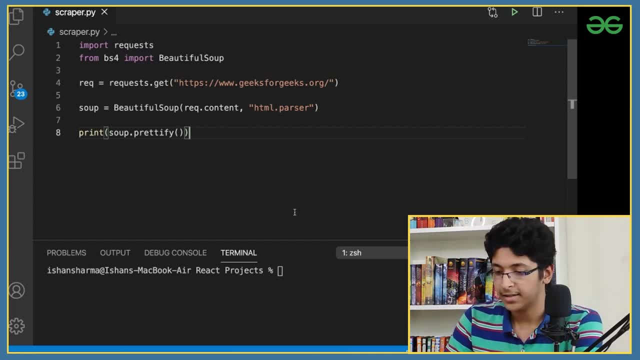 data. so i'll just save this and next i'll just go into my terminal and i'll just say python 3 and scrape paper dot py again. if you are a windows user, you will just have to say python, and that should work for you. all right. so what did we see here? we just got a bunch of data. okay, we got a lot, a lot, a lot. 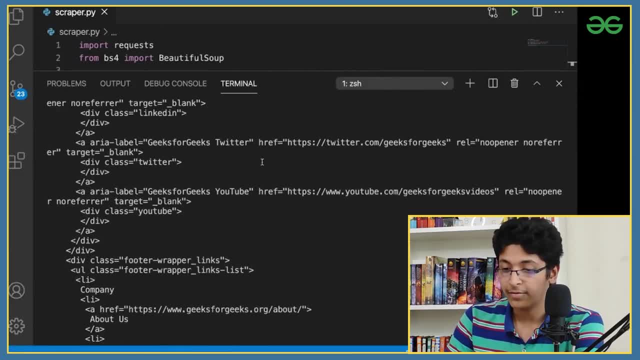 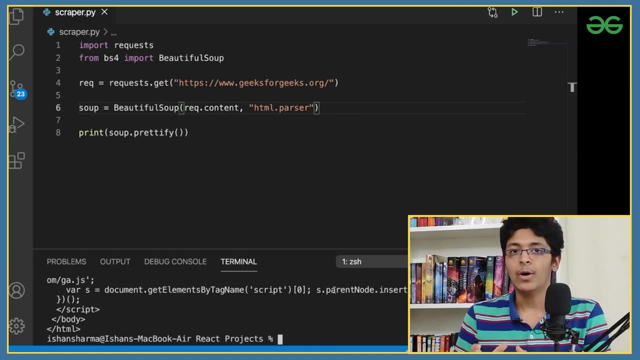 of data. as you can see right here, this is indented because we have used dot prettify, and if it would not, then we'll just get like a bunch of- you know, random gibberish. now let's try to understand how can we get specific elements from this thing. so the first thing i will do is that i will just go. 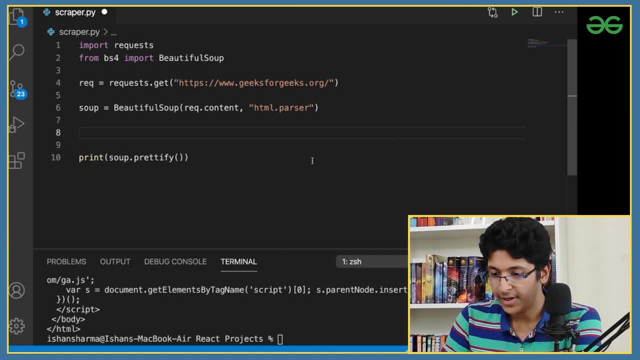 here and i'll just say: soup dot, get text. okay, let's just try to do that first of all. so get underscore text. that's what i will do here, and let's just close all the brackets. and now let's just try to run this. so let's run, and, as 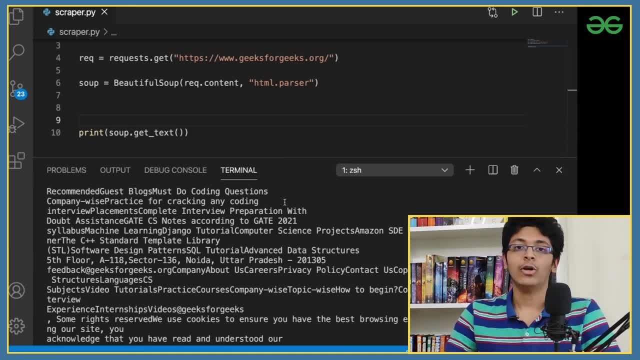 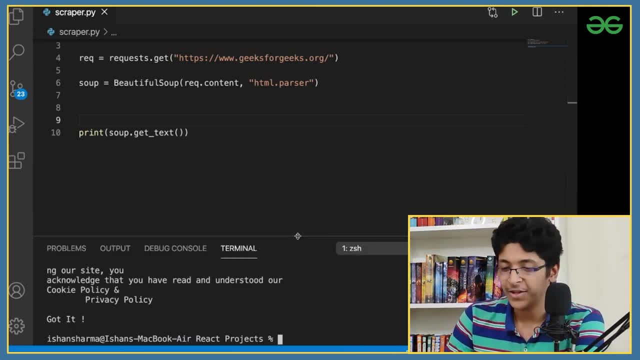 you can see, we get all of the text. so this is the text that you would be having in all of the elements that are inside of that. okay, so this is how powerful web scraping is. now. what else can i do? there's actually a lot of things that you can do over here.